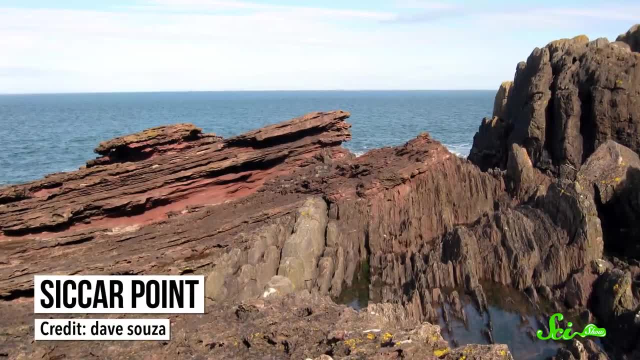 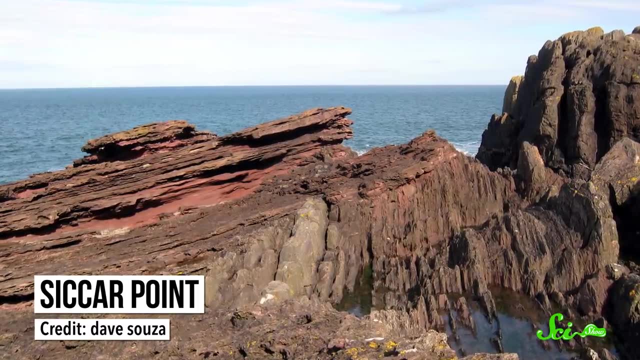 rock formations. The most famous of these discoveries was at Sickor Point, a cliff off the eastern coast of Scotland that features layers of red sandstone and greywack, a darker type of sandstone. The layers were sitting on top of each other, but they were also running. 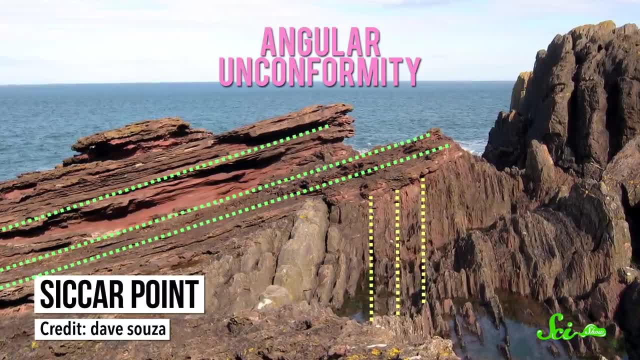 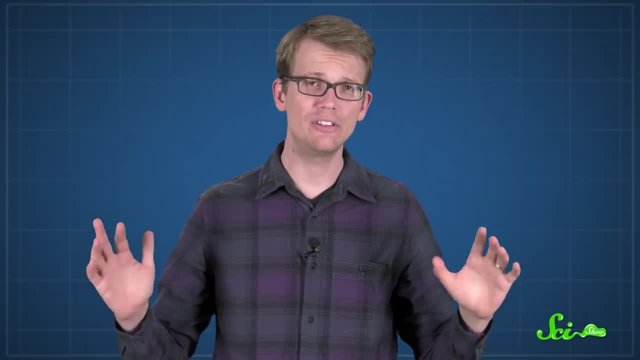 in layers perpendicular to one another, in what we now call an angular unconformity. He hypothesized that only great amounts of time and great pressure could have offset the rocks much longer than 6,000 years, And, as we now know, of course he was right This. 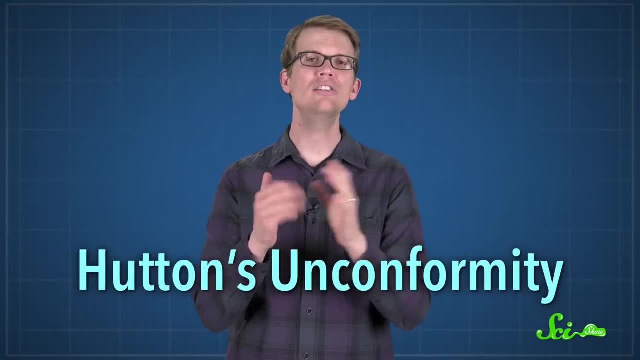 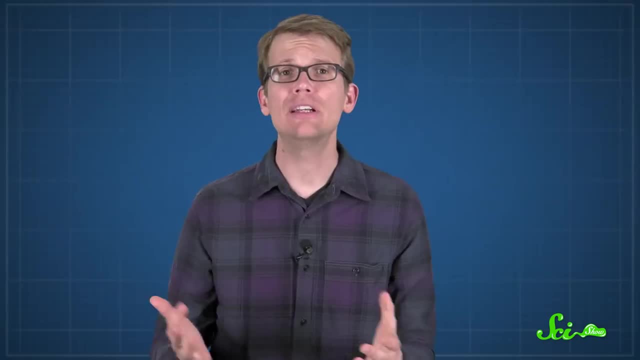 feature at Sickor Point and several others around Scotland are called Hutton's Unconformity in his honor. He also discovered that granite was an igneous rock rock formed by the cooling of molten lava. by observing tendrils of granite that had made their way into rock like sandstone. 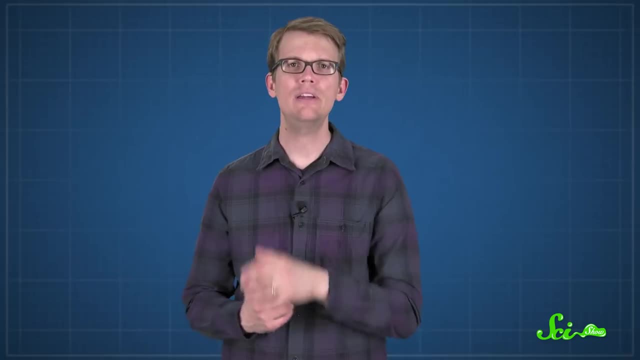 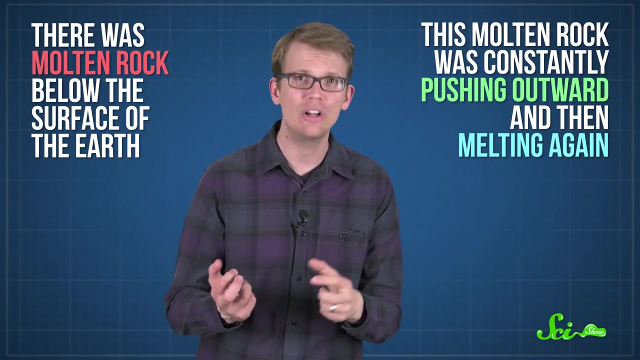 which he realized could only have happened at very high temperatures. Hutton believed that this was strong evidence that there was molten rock below the surface of the Earth and that this molten rock was constantly pushing outward and then melting again. He published his findings in a paper in 1788, but his theories didn't always. 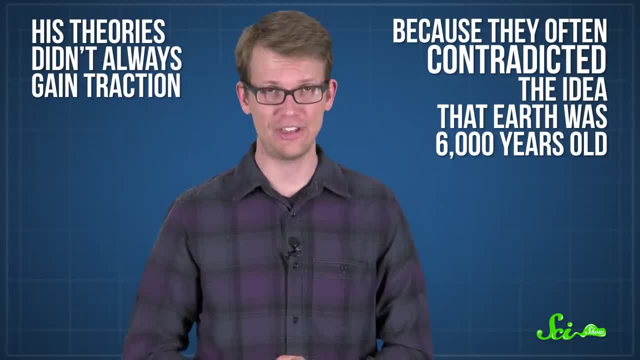 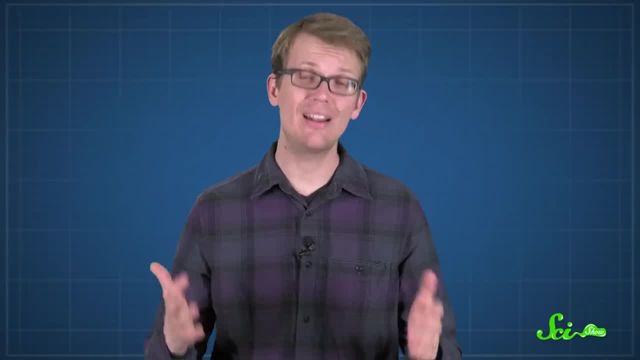 gain traction because they often contradicted the idea that the Earth was 6,000 years old, Plus a lot of other scientists' geological theories incorporated the Great Flood described in the Bible. Hutton's ideas did not, But a lot of his work turned out to be accurate. 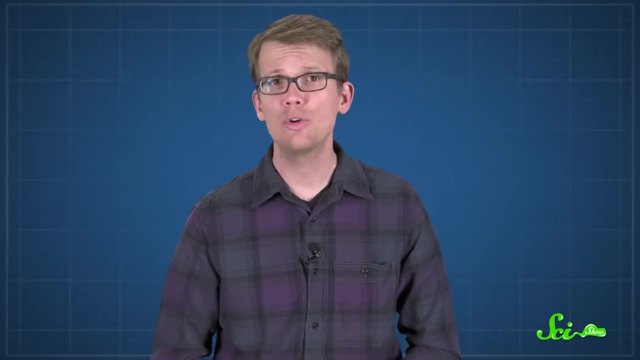 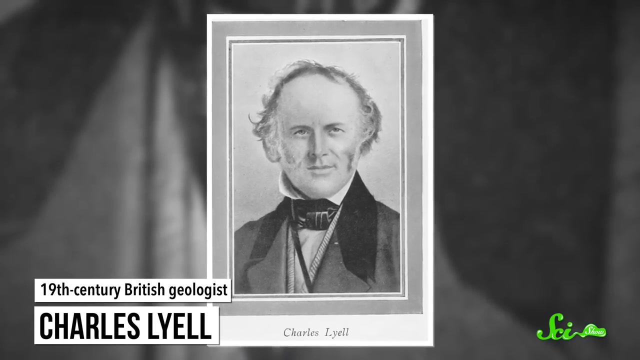 even though he didn't have access to technologies like carbon dating, which would have put actual numbers on the ages of rocks. Hutton also paved the way for future scientists, like 19th century British geologist Charles Lyell, to develop a theory called uniformitarianism. Uniformitarianism is the idea that the processes 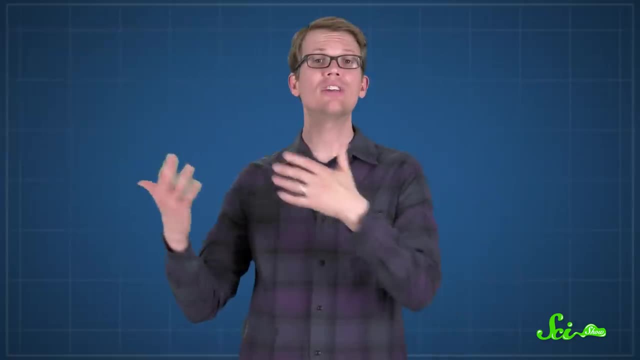 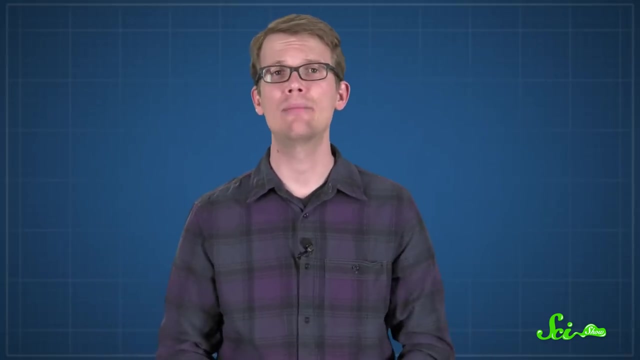 that shape the world now also shape the future. So what is uniformitarianism? Uniformitarianism is the idea that the past has shaped it in the past, So scientists can work backward and figure out what happened in the past By assuming that natural laws function in the same way across space and time. we don't. 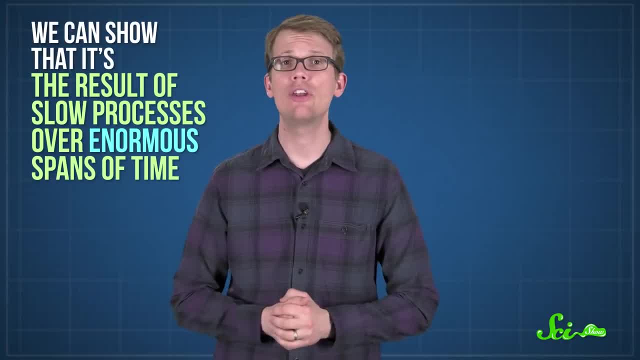 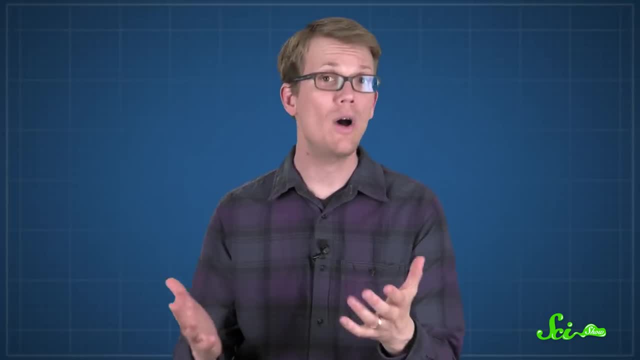 need major catastrophes to explain how Earth formed. Instead, we can show that it's the result of slow processes over enormous spans of time. Thanks to Hutton, the picture of our world got a lot more complex. He was wrong about some stuff, but many of his ideas helped shape geological concepts that we still use today. 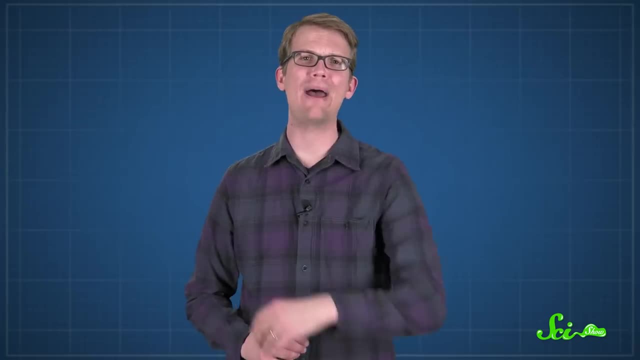 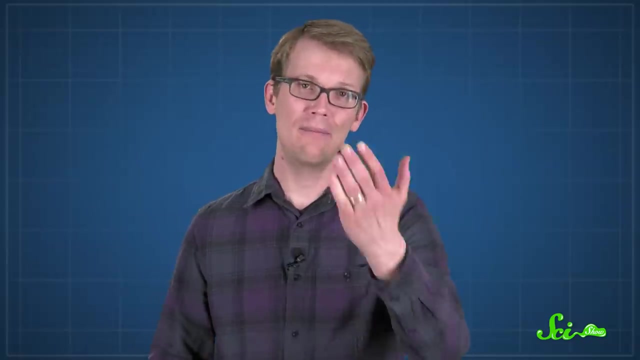 Not too bad for a guy who's famous for saying that the Lord should pity the backside. that is, and I quote, clagged to a head that will hunt stones. Thanks for watching this episode of SciShow, which was brought to you by our patrons on.